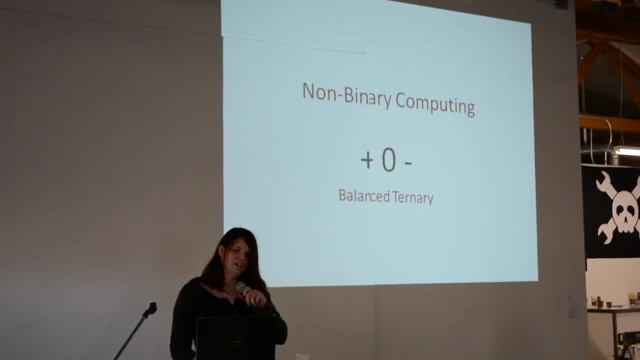 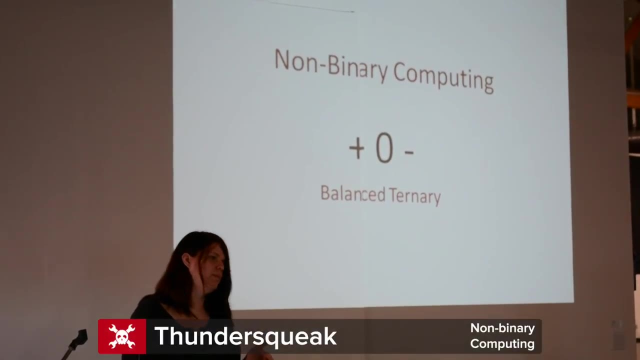 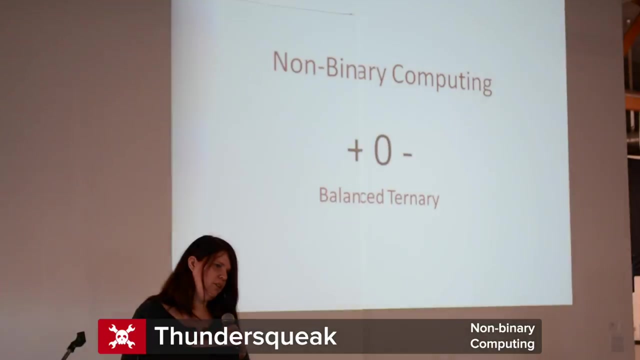 Well, thanks for that. Well, non-binary computing. What I'm going to be describing today is actually balanced, ternary, And what that uses is three states, where you have essentially a positive voltage, a ground state and a negative voltage to do the math. But what really got me into 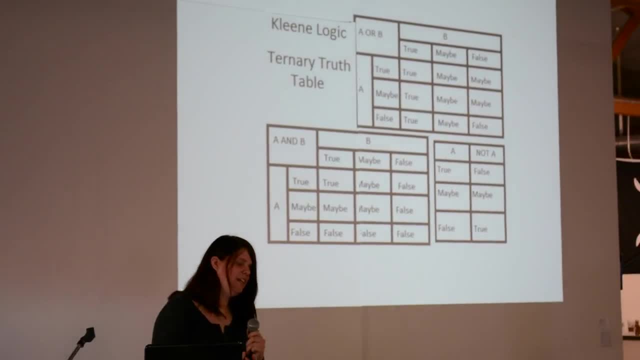 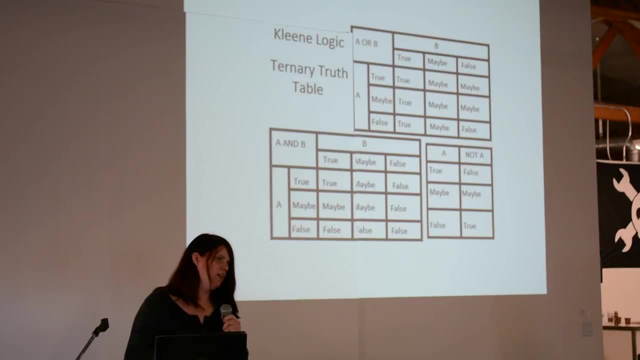 it initially is. I started looking at projects to do for the Hackaday Prize And I started looking at what people had done with different logic patterns. Well, for instance, the clean logic, which is more about how the human brain works as opposed to how a computer thinks. 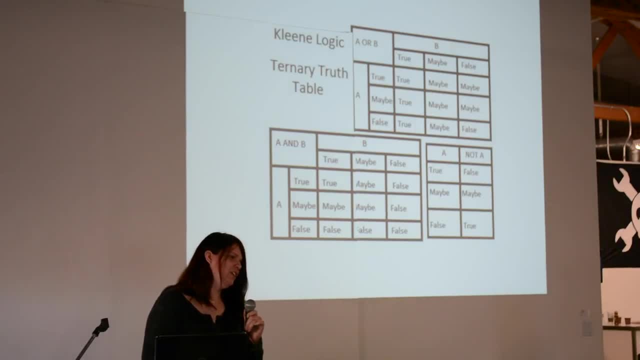 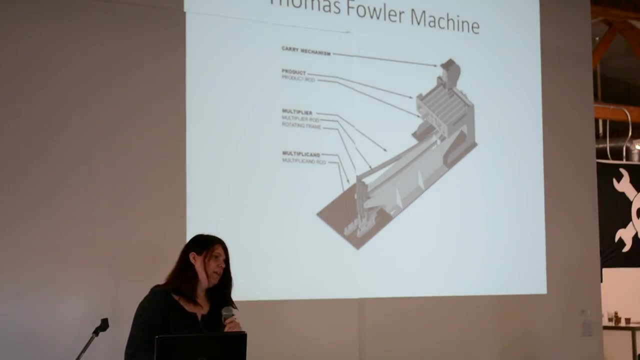 So I started looking at that. And it really doesn't translate all that well to doing arithmetic or anything like that, But it does sort of work out. So after a little bit of experimentation I started looking into what has been done in the past, And this particular device was invented by Thomas Fowler. 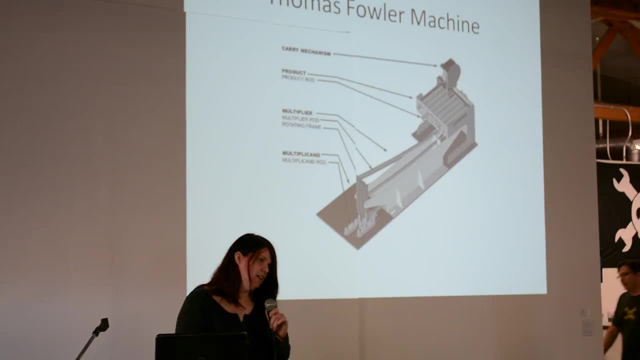 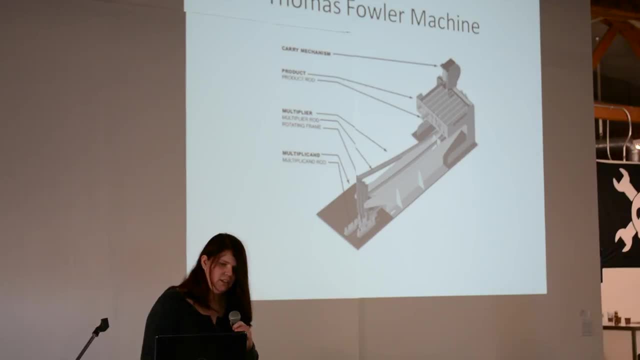 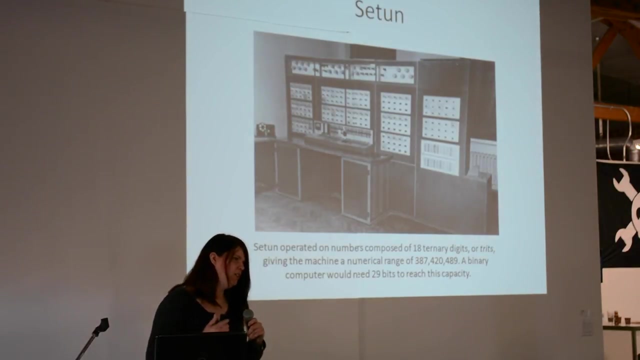 It had a carry mechanism. It calculated. It could do a multiplication division. He used it for doing logarithms and also calculating stuff for the church at the time. But let's see here. After exploring a little bit more I came across an old Soviet computer called the Satun. 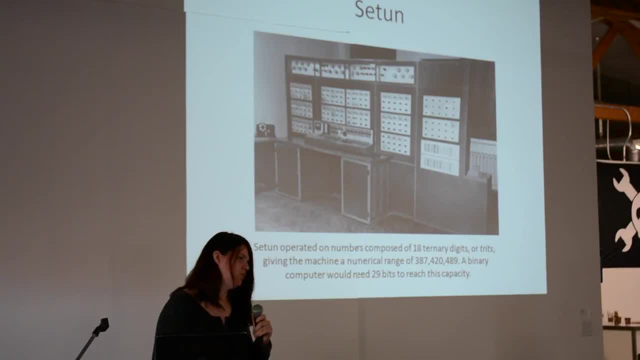 I'm hoping I'm pronouncing that right, But there's no schematics for it anymore, at least none that I could find. But it really opened up the door because, as far as ternary goes, it operated on 18 ternary digits, or what's called a trit as opposed to a bit. 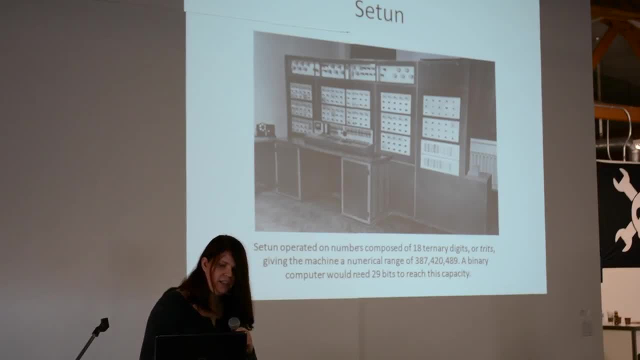 And if you look, it could actually calculate up numerically to 387 million something on a binary computer. Well, you take about 29 bits. It's a lot. It could take about 29 bits to do it, So it was actually a lot more efficient as far as how many components it used. The estimate is roughly about 2.5 to 2.6 times more efficient for each individual part, And they did this because vacuum tubes of the day were really hard to get to work stable, So they decided to just do it with a balanced ternary. 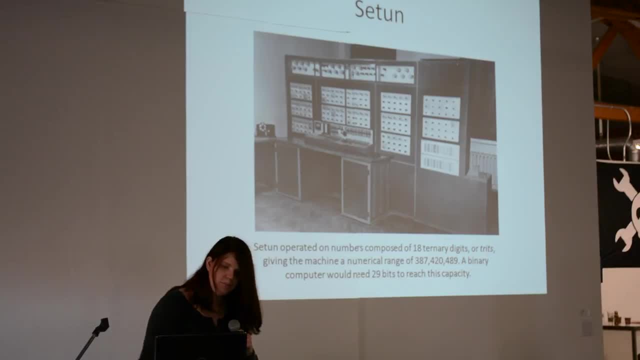 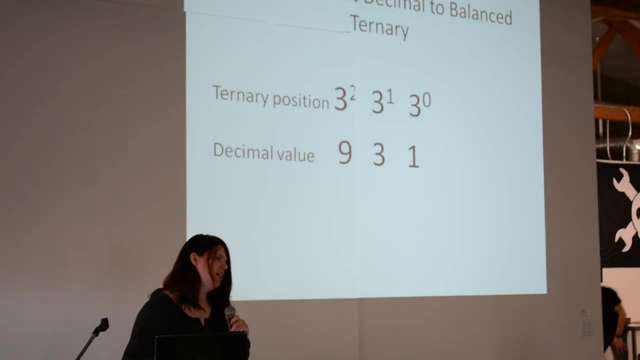 So you ended up with a machine that would actually be able to count, that would actually be able to calculate but didn't have to constantly be replacing as many tubes to do it. Unfortunately, it got abandoned in favor of binary machines as soon as the transistor came out. 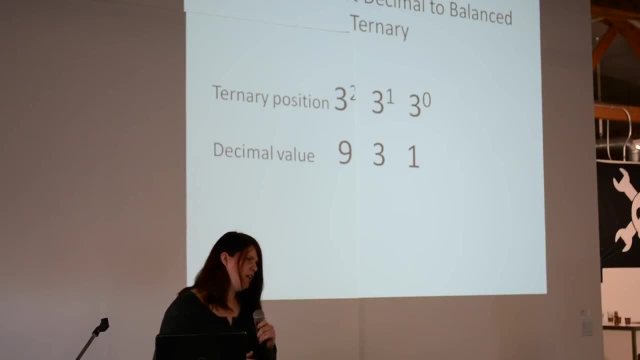 And that particular machine was done back in 1958,, I believe, and then there was a couple revisions of it after that. So what I was going to describe today was how to convert from decimal to balanced ternary and then show you a few of the calculations on how things 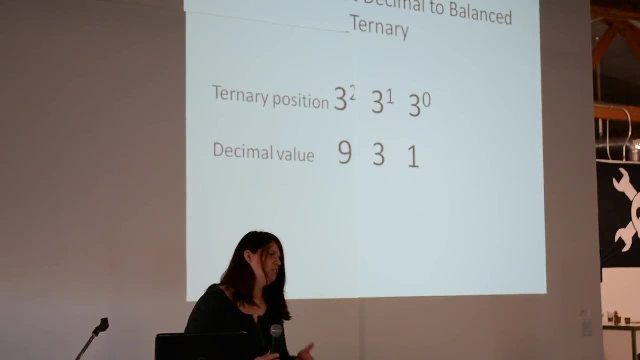 work before I go ahead and show you some of the circuits and what they do, because this really helps to understand how things function in the long run. But you're working on basically a base 3, and you're working backwards Instead of left to right. basically, you have your least. 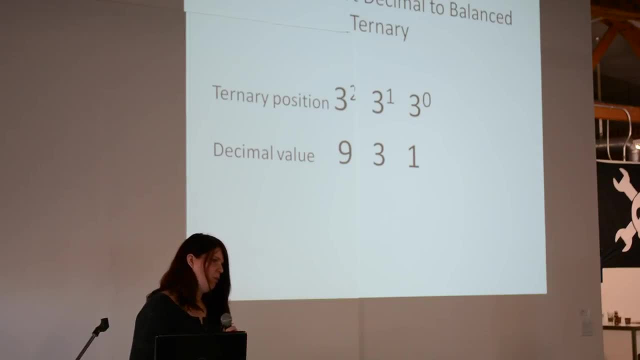 significant digit, just like you would have in binary Or a decimal system, but like 3 to. the second is 9.. And when you start doing conversions, when you look at things, for instance, well, to make the number 5, you put a. 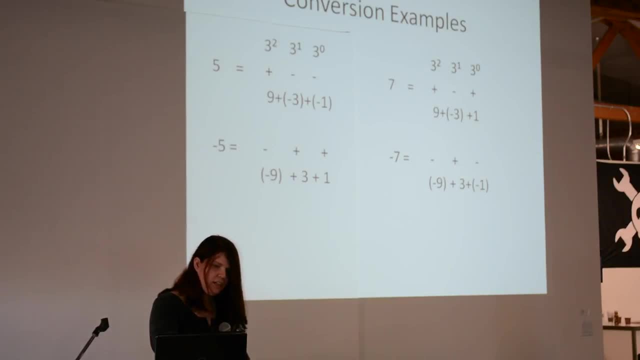 plus or a positive voltage, where the 3 to the second is and the other two are negative. What that basically represents is it's 9 minus 3 minus 1.. So you get 5.. And that's how a three-trit number system would work. 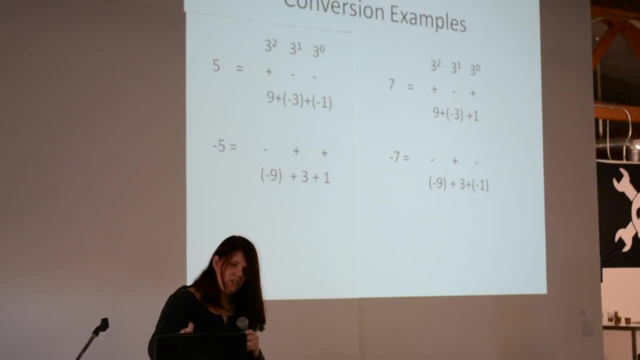 Conversely, if you want to do negative numbers, if you notice it's just kind of a reciprocal of what the original number was. So, for instance, you could do negative 9 plus 3 plus 1. And it works the same way for all the numbers. 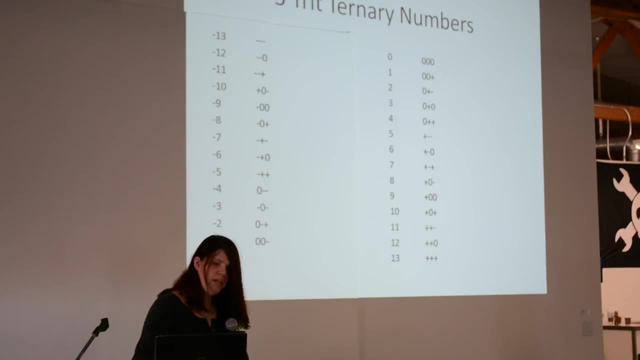 that are out there, And with three-trits it actually gives you a range of about 26 numbers. So that's negative 13 to positive 13.. So it's signed Basic logic table in case anyone's interested. But that's how you do the carries. 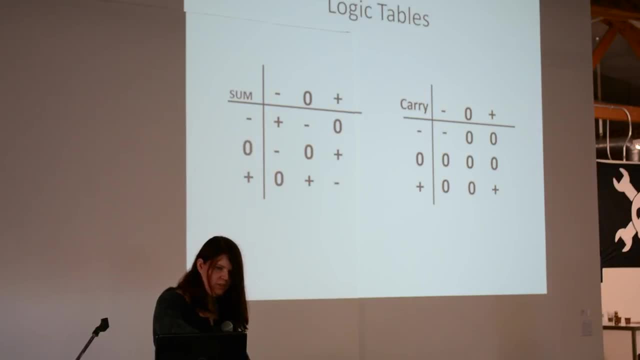 It's pretty self-explanatory once you get used to it. But if you have two negatives it's a positive, And two positives it becomes a negative And everything else just pretty much favors a non-zero state. And then on a carry bit you only have to. 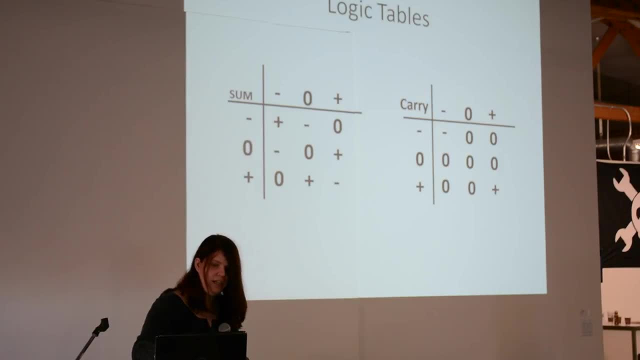 worry about the ands. So, negative and a negative, you get a negative. And a positive and a positive, you get a positive. But when you start doing things like addition, well, here I'm doing a 5 plus 6, just to show. 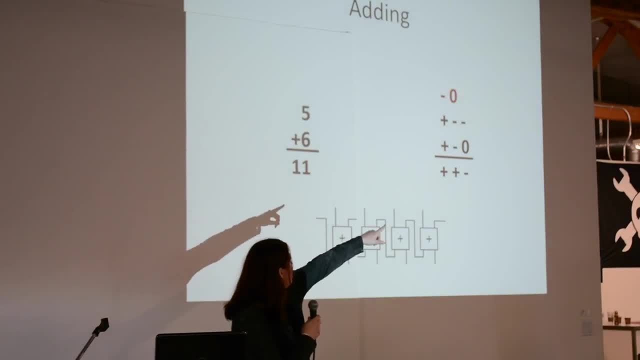 You start over at the far end where it has a negative over the 0,, because that's 5.. That represents 5, and that represents 6. And you end up with a negative And then you have a carry bit up there which is the 0,. 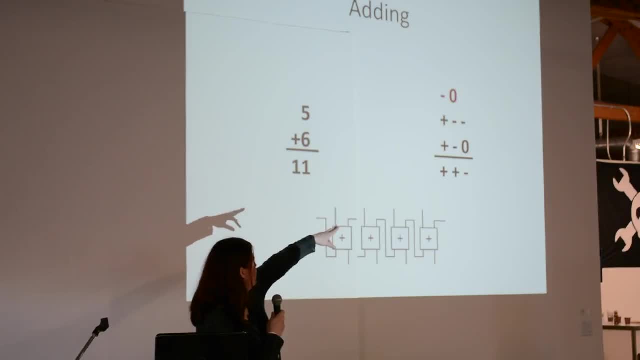 because it's not an and And it carries down. So you get a negative and a negative, which is a positive, And that has a carry bit of a negative up top, And then you take the negative and the positive and that becomes a 0, plus the positive is another positive. 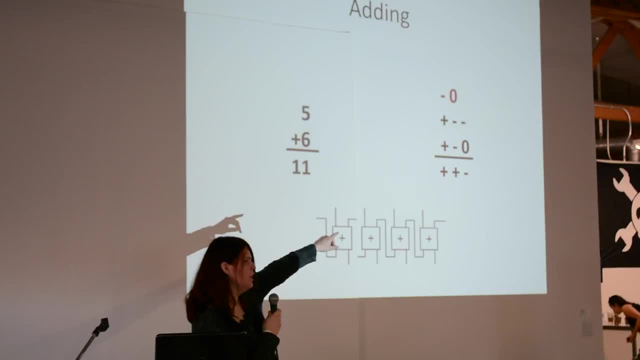 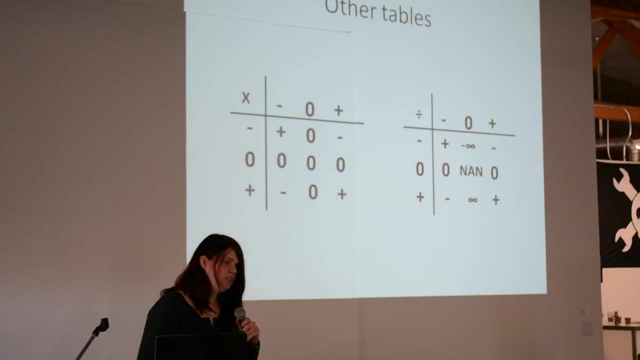 And if you were to add that up, it'd be 9 plus 3,, which is 12, minus 1.. And you'd end up with your 11.. And that's basically how ternary arithmetic works. You can also do a few other things. 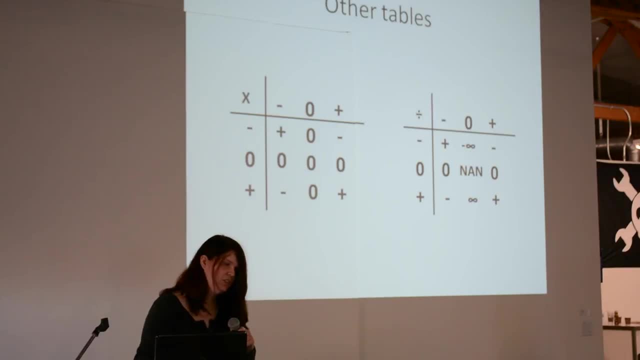 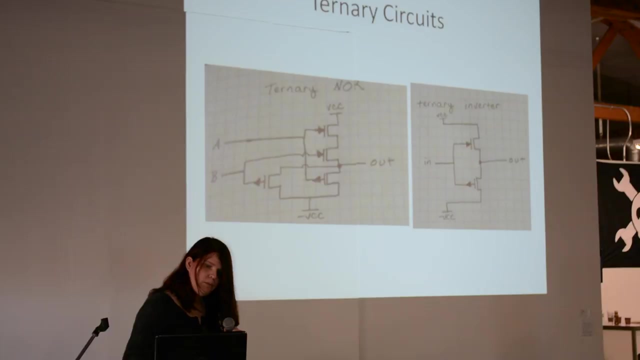 like, there's multiplication tables, division tables. I just kind of put these in here as a side note. So if you wanted to build a fully functioning AL arithmetic unit, it's actually pretty easy to do, just because it uses far fewer parts. 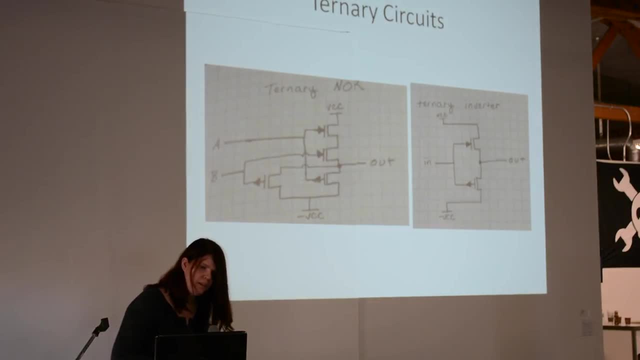 When I first started getting into it, I started looking at how to actually accomplish like an AND gate or an OR gate. I was thinking too much in the terms of how you would do it in binary And basically I ended up constructing out of some BS250s and some 2N7000 MOSFETs a standard building. 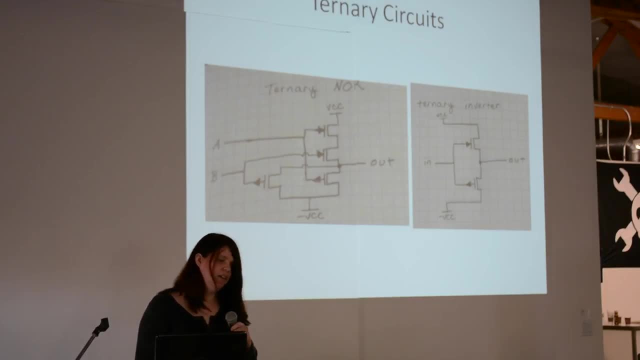 block, And that would be Basically you'd have. I'm trying to think how to picture this here. You have your AND gate, or your NOR gate, which basically is your sum unit, And your AND, or, in this case, an AND, is what it comes out. 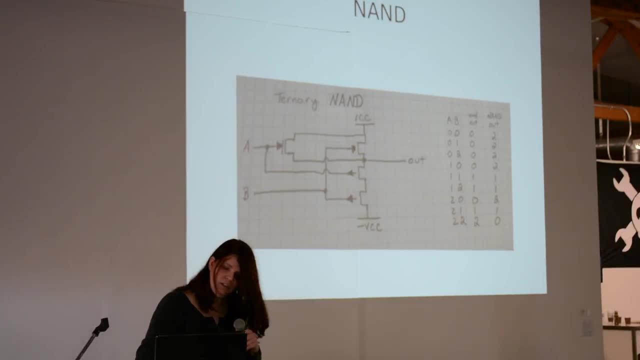 to becomes your carry. So, oh, the numbers on the side are exactly as you would for things to put in. There's your OR gate or your US gate to get rid of those counts Again. this is just an app, at least if you're. 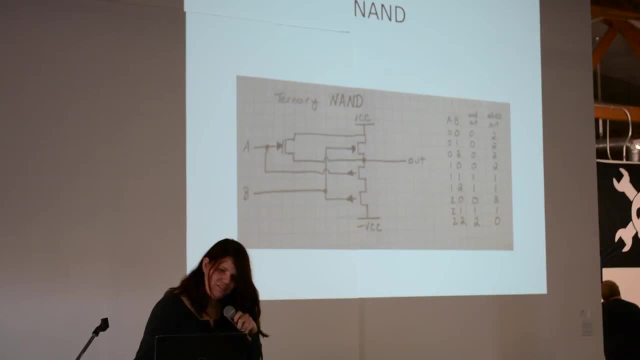 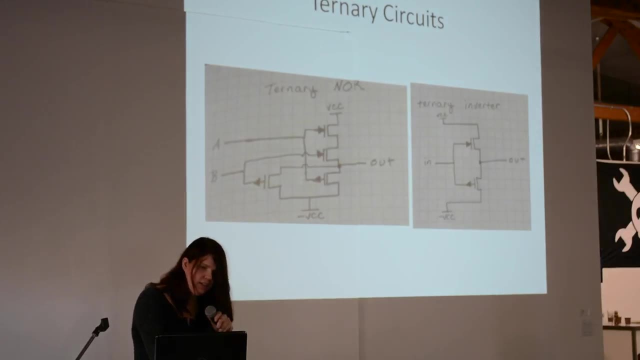 looking at an F abundance tool And you can sort of use prohibitive worshipping the error with the Ü gate. So again, no need to worry about this. I'll be simply saying what gave you an error out there. If you put in a 1, you'll get, or if you put in a positive, you'll get a negative voltage out. 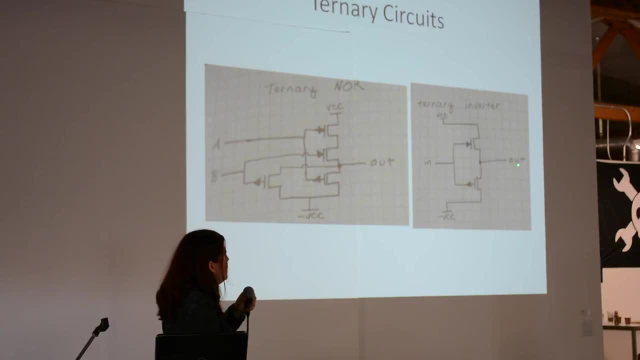 If you put in a negative voltage, you'll get a positive voltage, But if you put in a ground state or a zero, it just stays zero. It doesn't actually do anything, which essentially satisfies the requirements for the AND table on the carry. 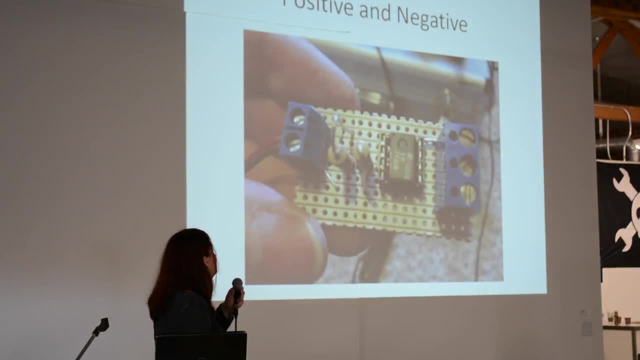 And so I started building the circuit up. This is just a. I was doing a splitter Instead of using two resistors to split for a positive and negative rail. I just did kind of a floating ground And I just put this in because it was part of the process. 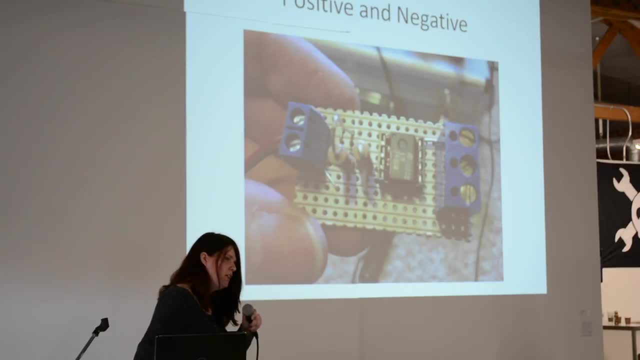 But that used a 741 op amp, which is a pretty interesting circuit if you're needing split rails and you just have a 9-volt battery sitting there. If anybody has any questions on that, I don't mind. And then going through and just breadboarding stuff. 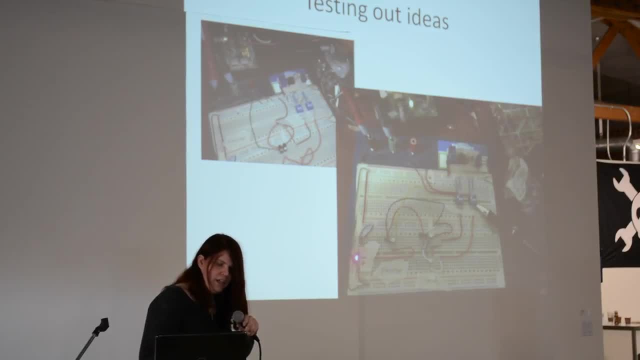 So eventually I went through and I decided to start building this stuff up. And here was one of the experimentations beforehand And I was just doing a voltage divider circuit using MOSFETs. But here, if you noticed, I have a- let's see, that's a negative- and a negative switched on. 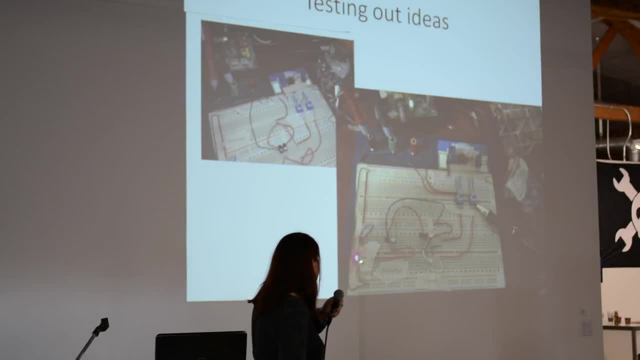 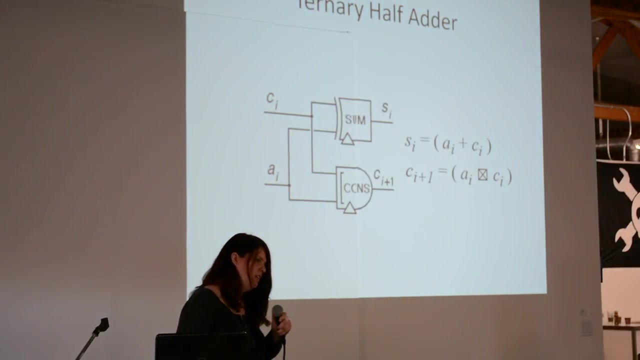 And then I'm running it through an inverter Because it was a positive And so I'm getting a negative out. So that's actually working properly. And that was just basically part of the design process. So then I started going into more work to see if I could design a functional arithmetic unit. 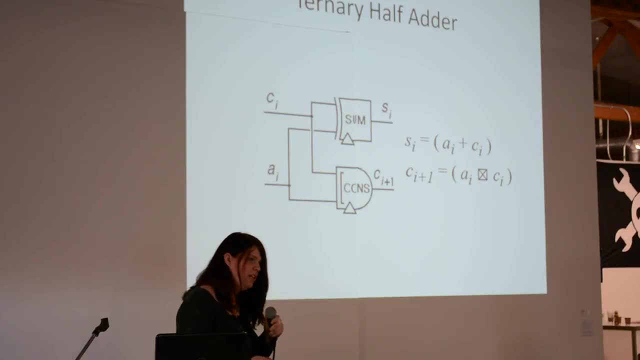 And well, your basic half adder. if you're familiar with binary adders or binary half adders, it actually it should look pretty familiar to you. So, basically, you have your carry in and it sums it up, and then you end up with your other carry out. 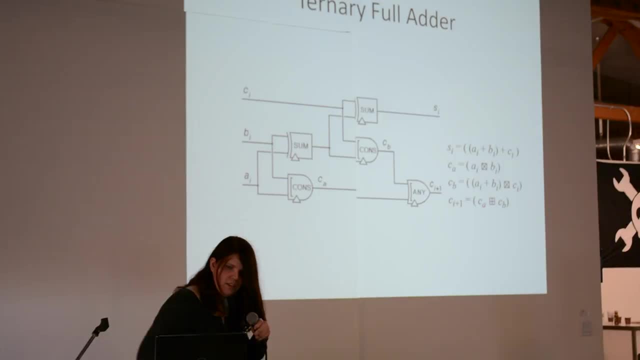 So, based on that building block, I went over to a ternary full adder And after you start doing this, it just kind of. you can basically use this circuit If you're familiar with a what a ripple? kind of like a ripple. 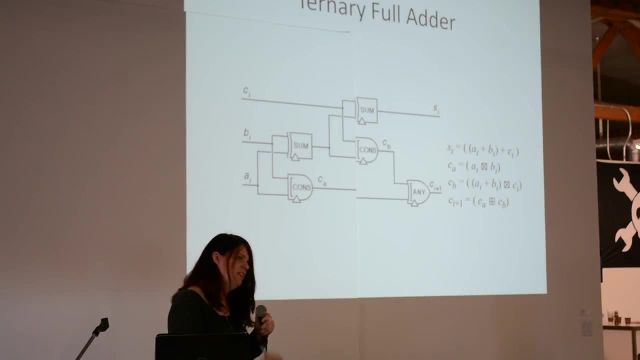 God words on the tip of my tongue now. Hmm, Yeah, ripple carry, That's what I was looking for. But basically, if you, it uses a pretty standard circuit, So it's very familiar, if you're familiar with binary ALUs. 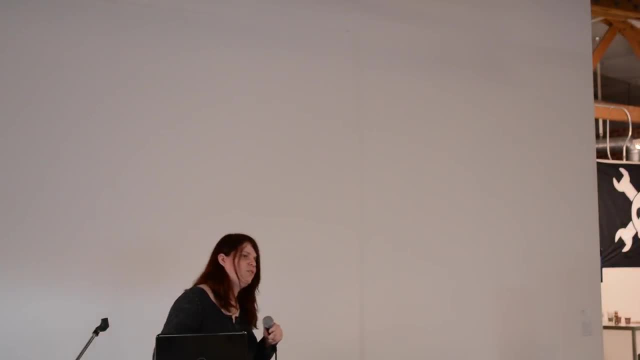 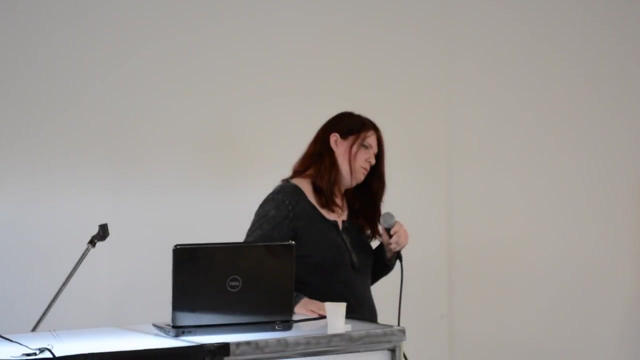 So let's see, That's pretty much all I have for slides, Probably running really short on time because it's something that I wasn't. I'm sure I don't explain, But if anyone has questions, When you were at the prototyping stage, how hot did your chips get when you were trying to do it for zero? 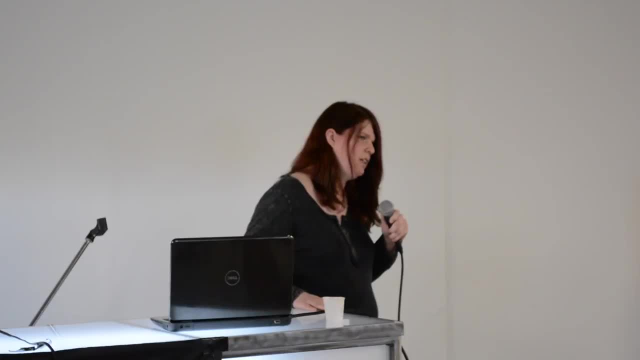 Actually it didn't really get hot at all. I was working with very little current and pretty low voltage. I just made sure I stayed within the threshold of the chip. But I mean based on the construction bed or it was like the old devices are halfway off. 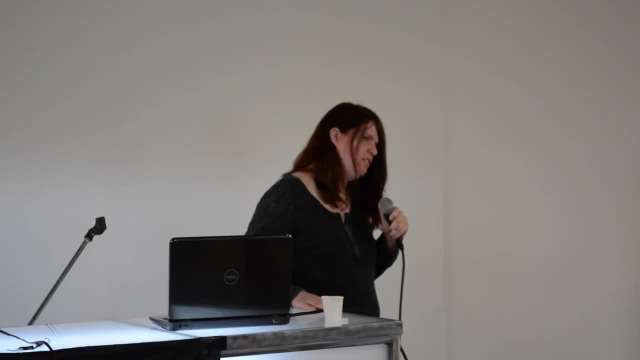 They are, but I was staying below what the or I was staying within what the chip could handle when I was doing it. Why didn't you sign both of them out? It's kind of the same thing. It's just really funny how you were thinking about it. 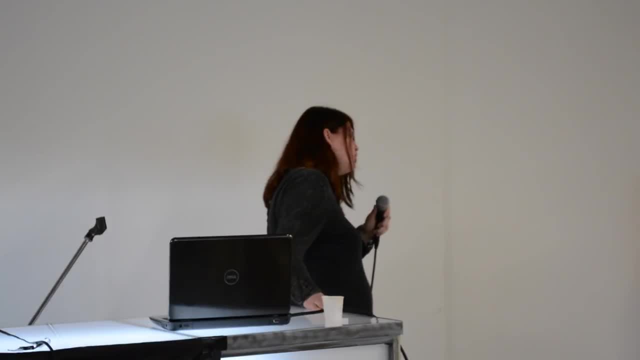 Mm-hmm, It's like you signed it. Yeah, I actually started looking at the doing an unsigned Or an unbalanced ternary system in the beginning, But it decided to go with the balance just because as far as the voltages worked. 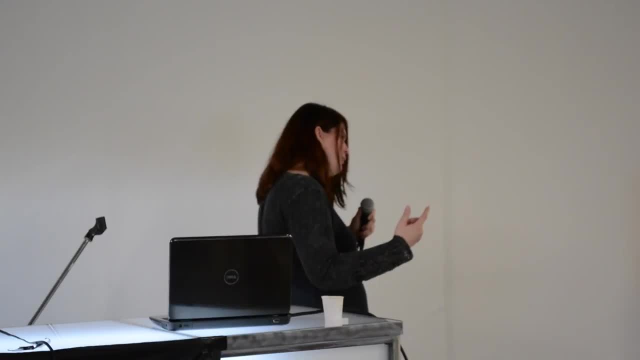 it was a lot easier for me to mentally wrap my head around and work with The other one just got a little on the confusing side. as I was trying to build things up, I started getting odd results. It's interesting that you go that way. 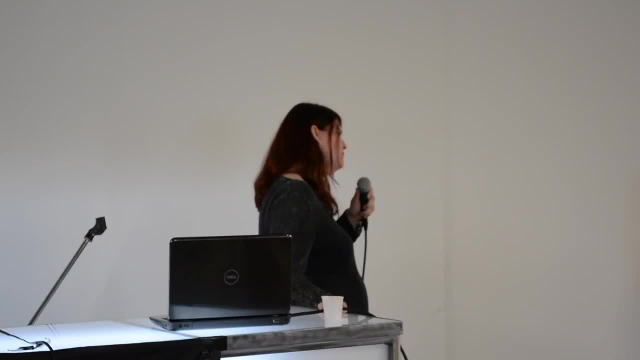 She says: what about when you start out and apply a new system? You're thinking in an unsigned way. It sounds interesting, It's very interesting, Yeah, well, also, when you're working with a balanced ternary system, you end up with a few oddities, as opposed to an unbalanced system. 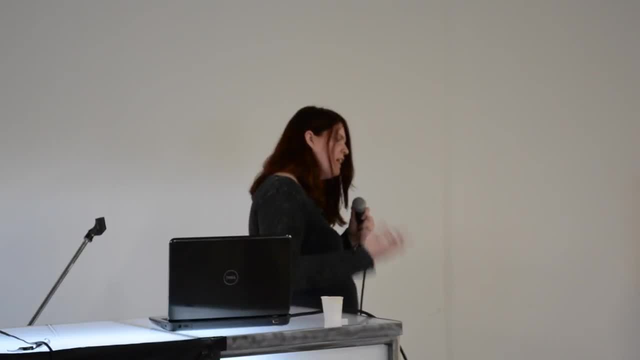 For instance, when you're doing an increment on a binary system, you're actually you can only increment. However, on a balanced ternary system, that same circuit can also de-increment. So it was basically: you're basically getting two functions for the price of one. 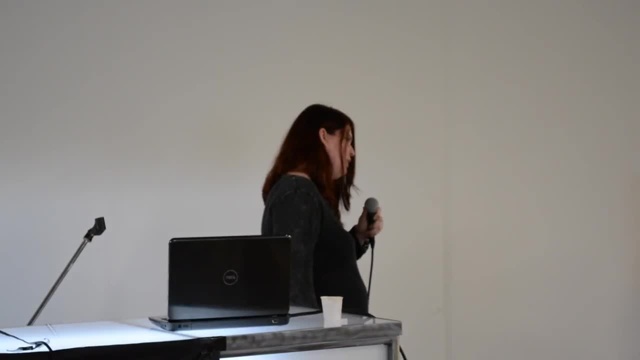 because you could start counting backwards and start handling negatives and everything else, And that's where you could kind of just kind of keep adding up. I have started looking into: was it a predictive carry instead of doing the ripple carry? And that's basically where I left off with when I flew down from Alaska. 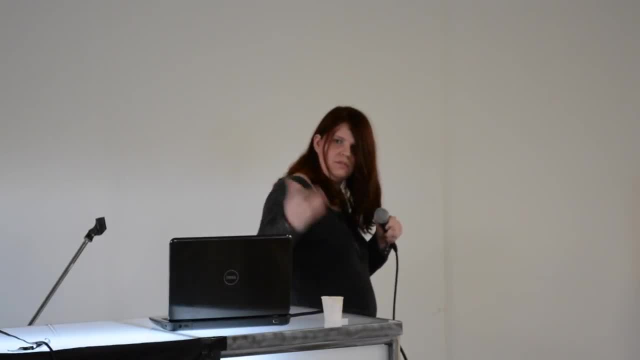 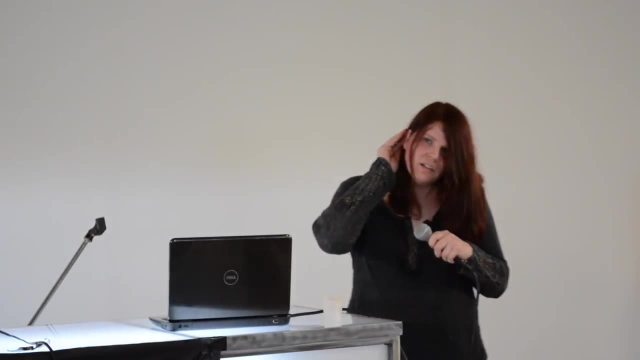 So Any other questions? Can you talk a little bit more about the increment and de-increment in the same hardware? Is the increment and de-increment in the same hardware? is there like an external pin that changes what you're doing? No, not at all. 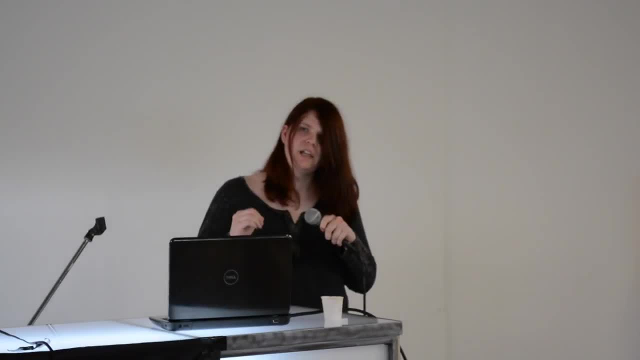 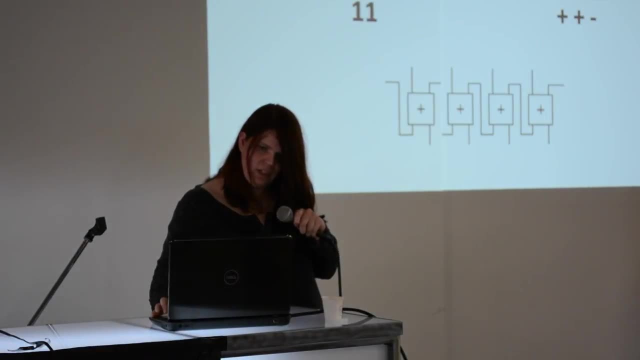 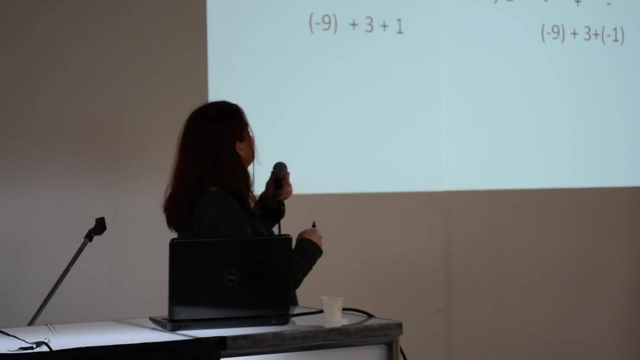 How does it know whether the increment is? Oh, by it being a positive or a negative voltage Here. See when you're doing the math here, by, basically, when you change a, for instance the three's place, to a negative. 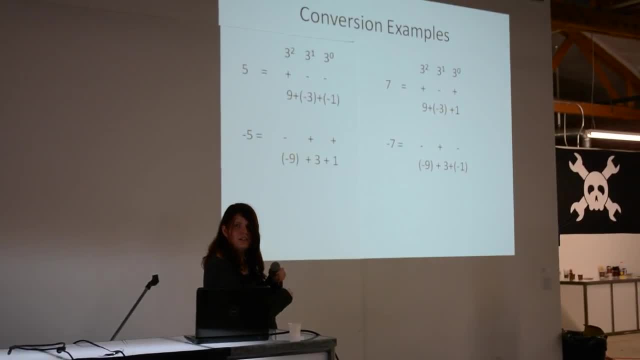 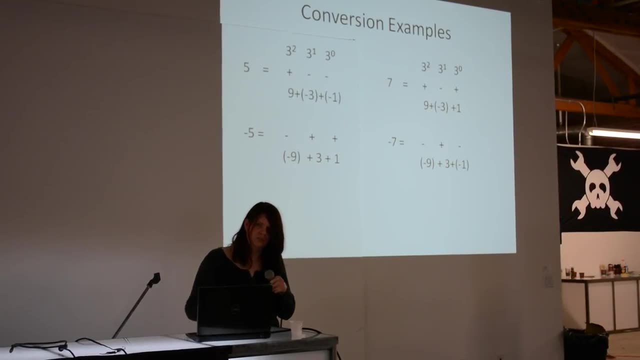 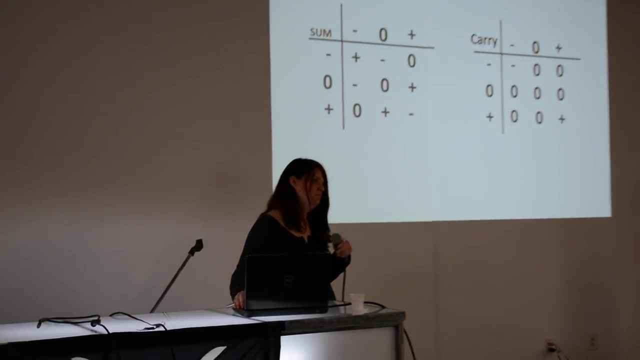 it actually will de-increment a one right there As opposed to always incrementing. There's no real toggle to it, It's just it's kind of inherent in the design. Okay, Um, Is there like a bundle, A set of trits? 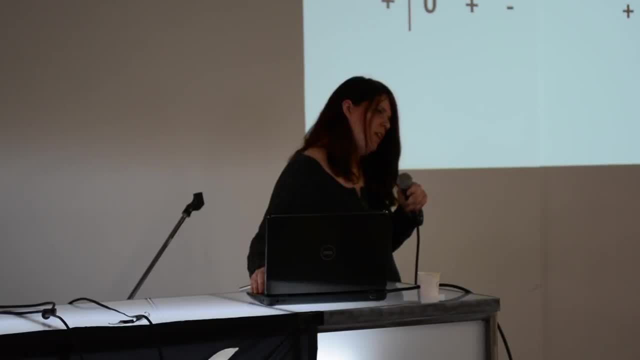 Like: so like eight bits is like, is there like a trite? Uh yeah, Is it a trite? You know, I've never looked that up. No, no, Can you tell me what that is? That's really cool. 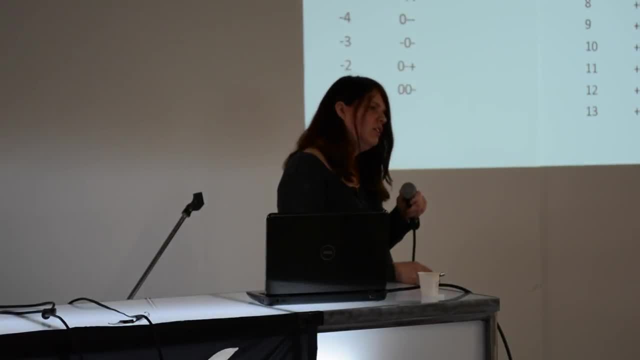 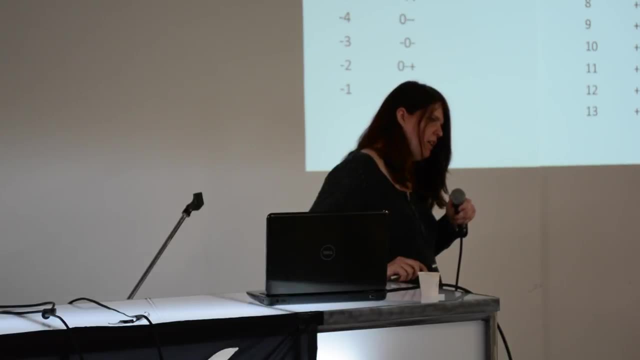 Like: is it going to be a nine and that's a trite? Well, the originals, like the Saturn, was using 18 trits. Oh, okay, And that's where I could count up to. uh, uh, yeah. 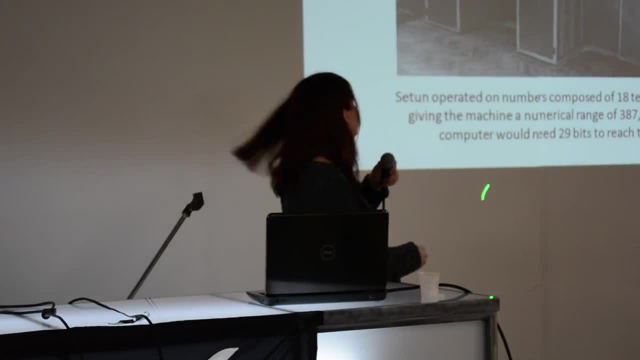 Yeah, 800 and yes, 837,. uh, million as opposed to uh. you'd need 29 bits to do the same. How much, uh? what did you say? for example, the clock cycles when you're doing your let's. 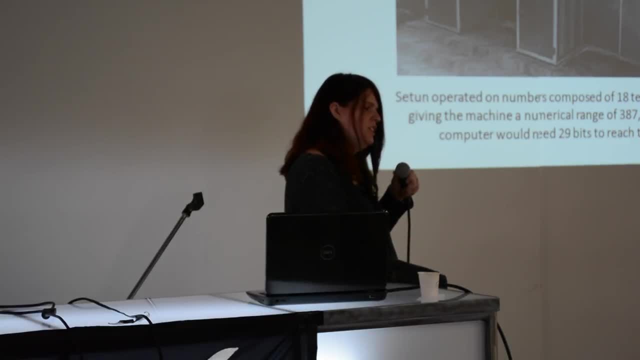 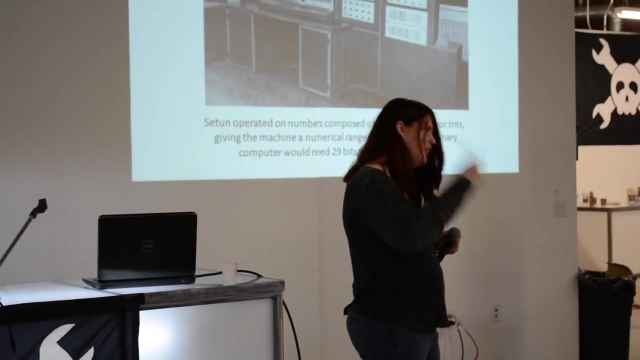 say: you know binary, You know I've not really done the math on that one. Uh, run that by. I actually can't hear. 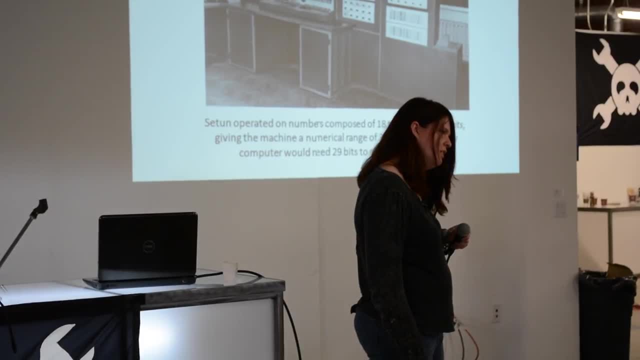 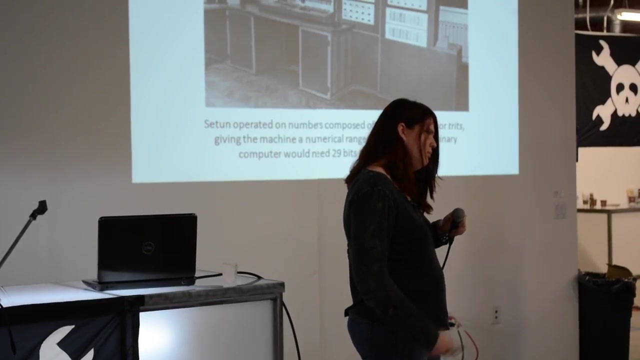 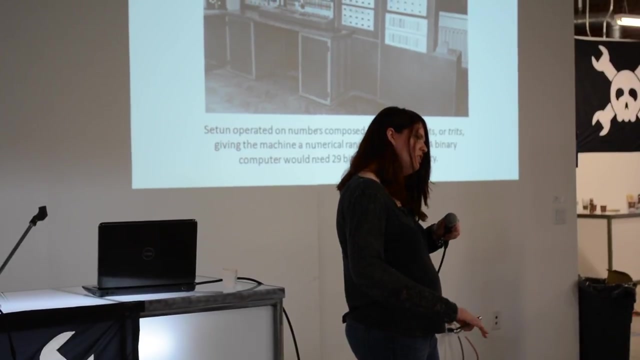 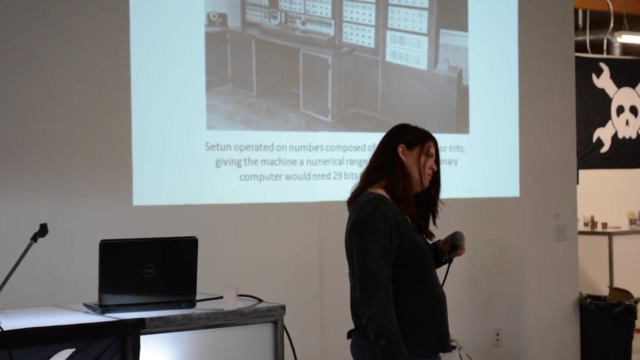 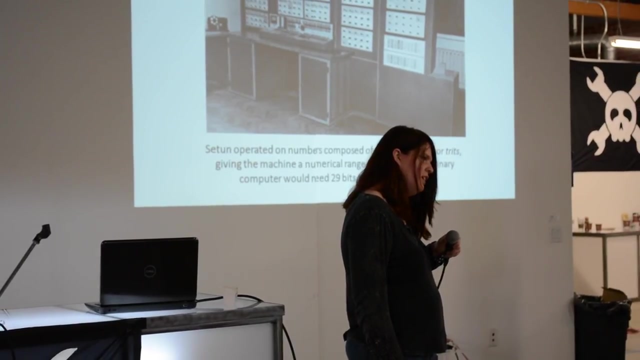 Yeah, I actually considered doing that. I was looking at using the PIC micro originally to kind of work as the controller for it. 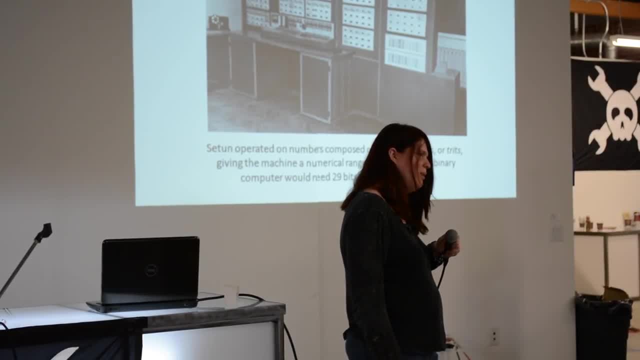 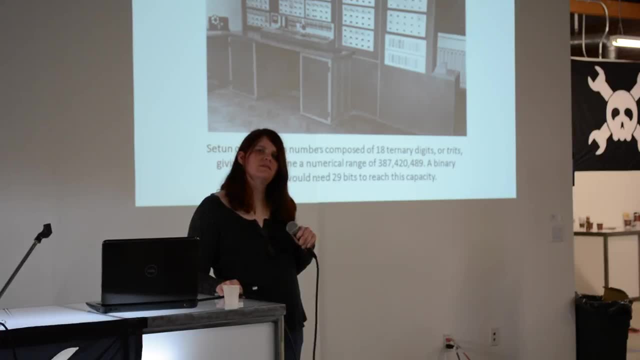 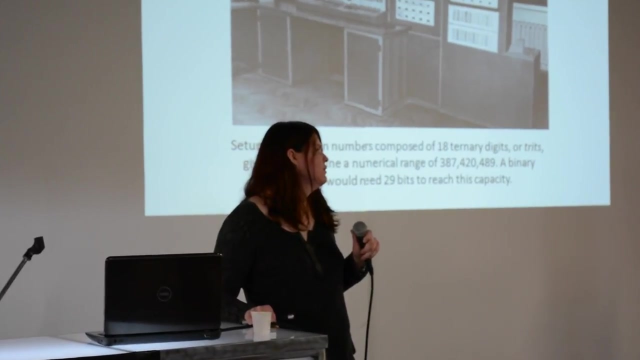 And then I basically ended up stopping because I was doing this for the Hackaday Prize at the time. Yeah, Yeah, Okay, Okay, That's it Okay. So let's move on to something else. Yes, Yeah, Yeah, yeah. 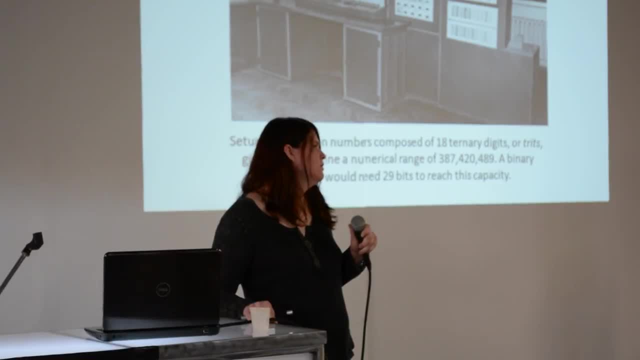 Okay, Yeah, I think that's. that's a good question. Yeah, Yeah, Yeah. I just wanted to point out, you know we're talking about the Yeah, Okay, Yeah, Yeah Yeah, I didn't quite catch what you're saying. zero point stability. oh okay, and it's. 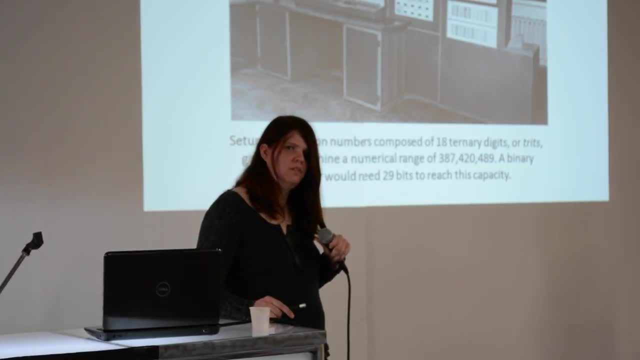 ground, it just stays ground. yeah, it will. sorry, I actually have a hard time hearing you for some reason. I actually didn't notice that, at least not that the scale I was working at- yeah, no, it was more at the time, it was more of a let's see if I can do this thing. so 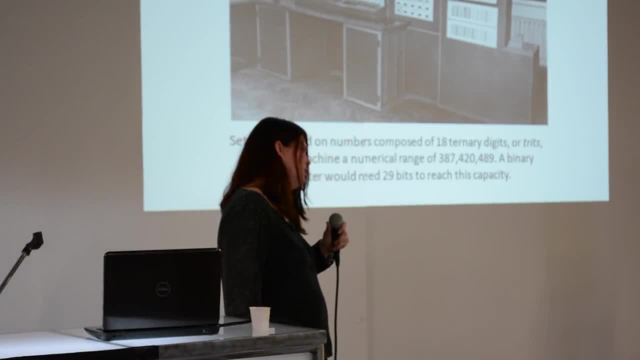 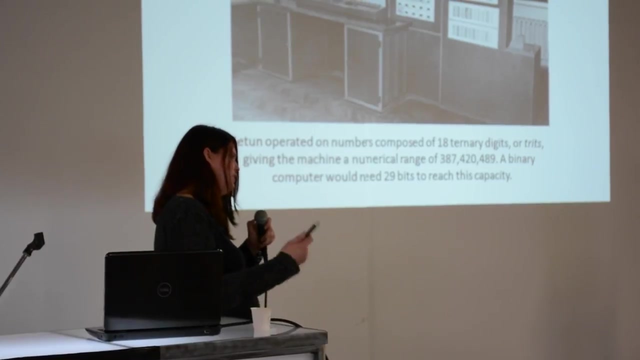 yeah, but that was. it was basically a let's see, see what I can do as far as building. I was thinking about building machine originally and I started looking at like the z80 in the 6502, and then I was like, well, let's build something else. 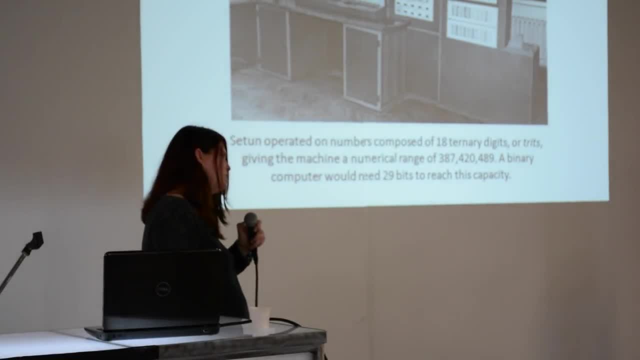 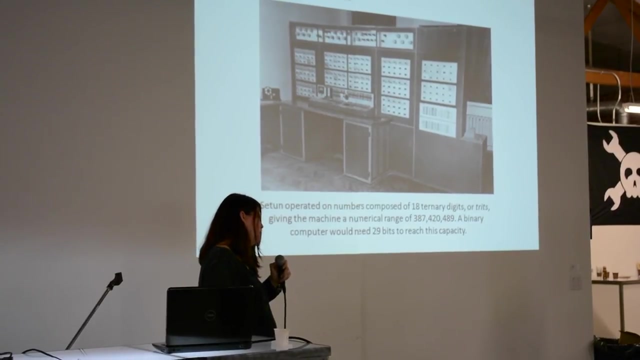 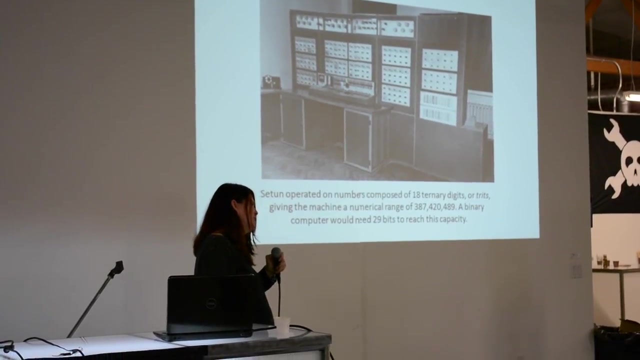 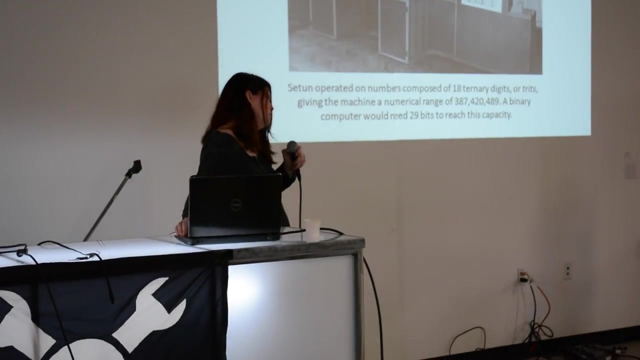 and so I started looking at other people's projects and No, they used tubes, but it was a pure, balanced, ternary system. Unfortunately, the schematics for it are still either lost or classified, so they haven't given them up yet I have. 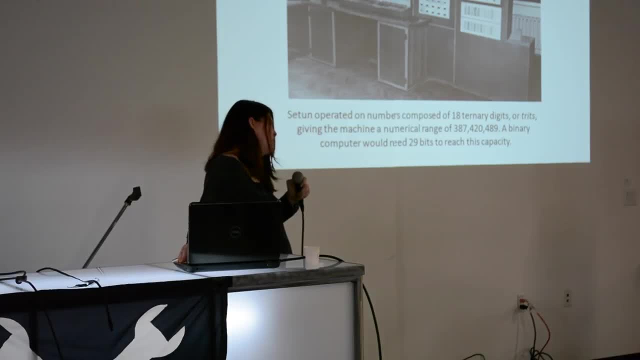 That was the first thought I had. I got a Cyclone II FPGA and that was the first thought I had was to start looking into actually implementing it that way. Have you looked at universal logic gates that are managed in the works? You know there's like 17 of them. 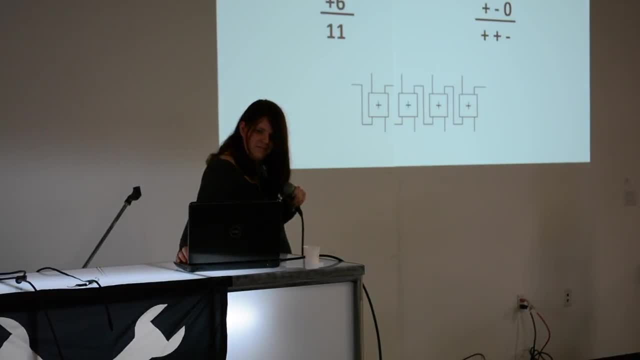 They actually need to be managed. Do you need to say some philosophy? Well, as far as looking at anything beyond the basic gates that I looked at, no, I got that working and then I kind of continued. Did you have any thoughts?